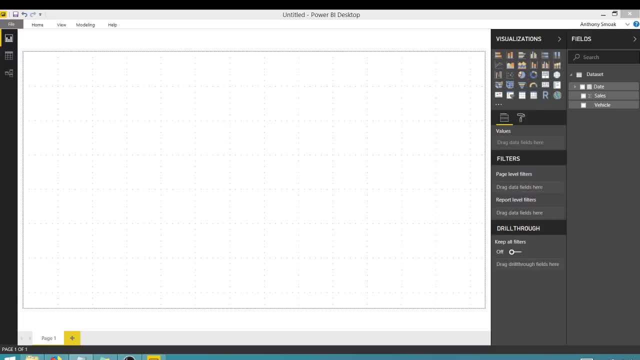 All right, Thanks for tuning in everyone. This is Anthony Smoke. Go ahead and check me out on anthonysmokecom or follow me on Twitter at Anthony Smoke. Today we're in Power BI switching it up a little bit, switching over from Tableau to Power BI here, So you know. 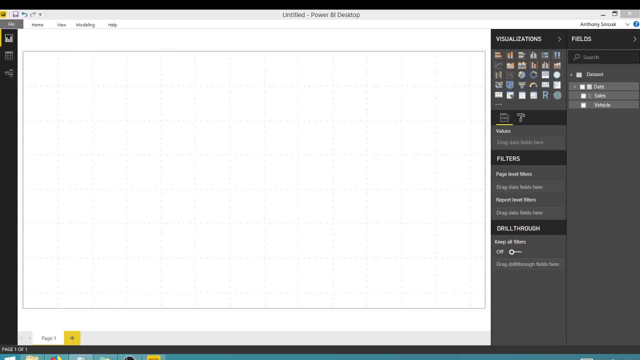 I believe if you're going to learn a new tool, you should know how bar charts work right. That is the basic best practice for visualization. So there are some things that you know I was trying to do while creating a visualization. I needed to know how to get a percent of total. 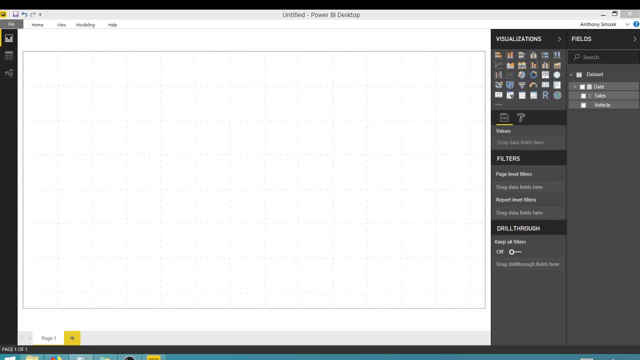 on my bar charts And you know I had to skill myself up to figure out how to do that, Did some research And, as is my MO, I wanted to share that. So let's look at the data here. So we're. 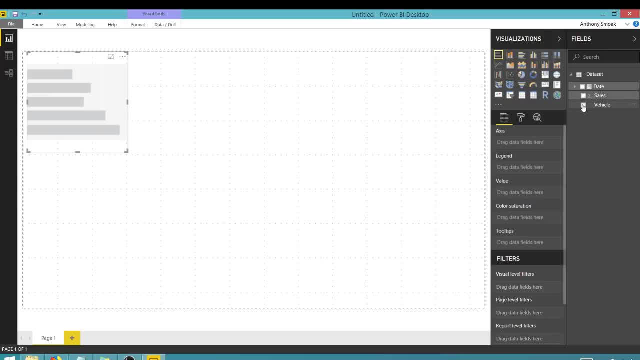 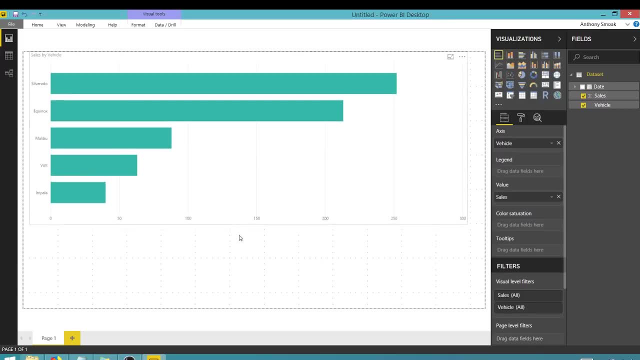 going to bring in just a basic bar chart. I'm going to bring in let's see vehicle and sales, And so what I've got here? I've got a fake data set And we're looking at uh, uh vehicles and we're going to turn on first of all here. we're going to turn on our 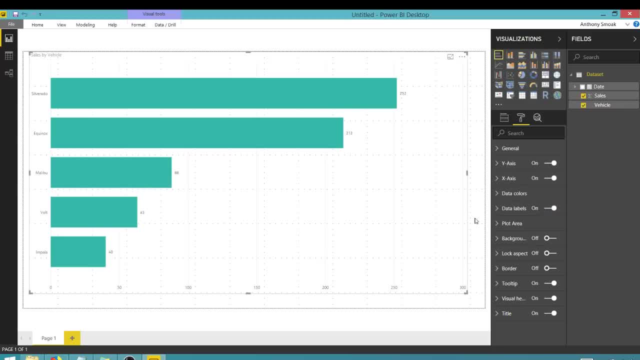 data labels. That's how you do that in Power BI. Um, as you can see, I've got a vehicle here and we have the number of sales. So, very basic, this is fake data and I'm using a GM vehicle. shout out to a Detroit, Detroit steel there. So, um, let's do this. first, Let's do a little. 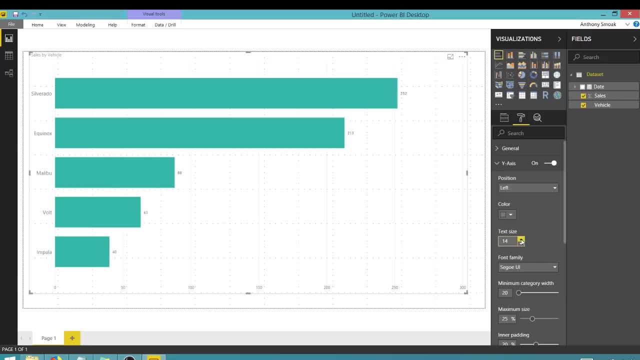 bit of formatting. Uh, just going to turn The font up here on the Y and on the X. let's increase that, uh, the tech size on the axis, and uh, on the data label. we'll do the same thing. So you have to know where all these 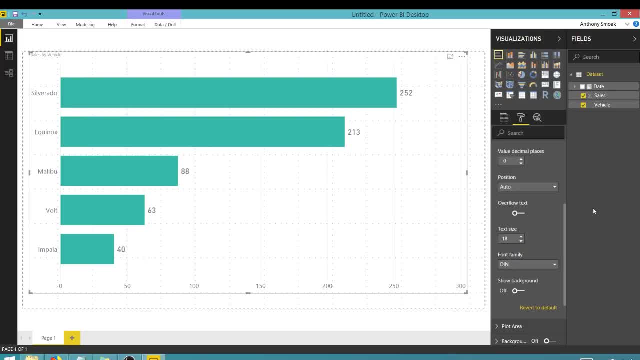 options are in a Power BI, uh, when you start using a- uh, a new tool here. So so, as you can see, I've got vehicles and I've got a number here. So what I wanted was I didn't want just the- uh, the number of sales here. I wanted a percentage. 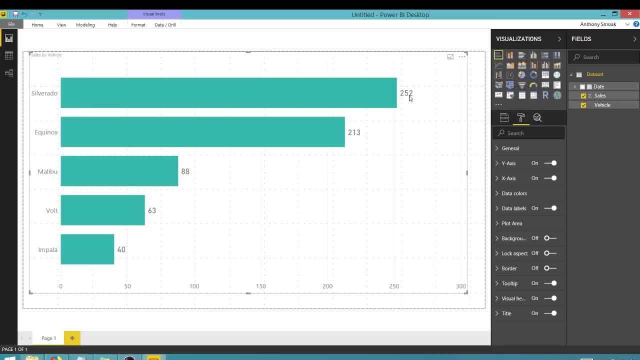 total, right. So this uh, Silverado sales represented how much of the total. So you know a tableau. this is a quick table calculation and you're done. but you know Power BI. uh, you have to, um, go through a little bit more, uh to get that to result. 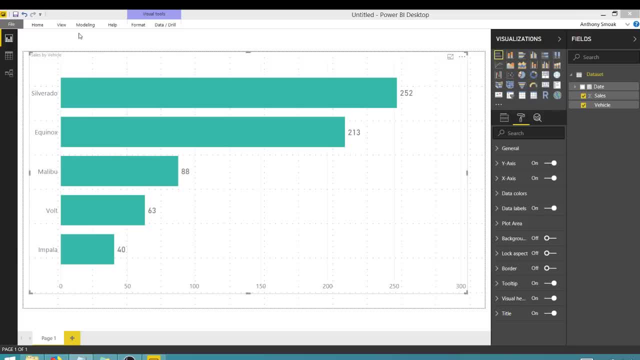 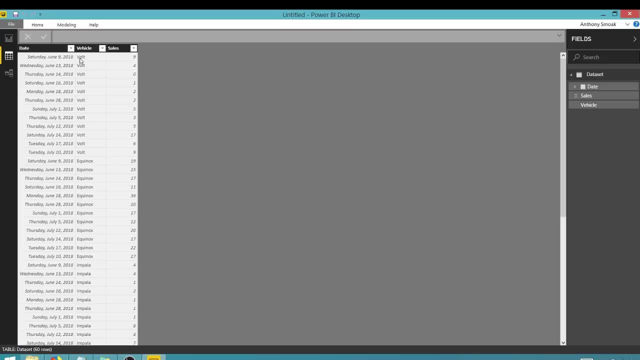 So, uh, what I'm going to do here is we're going to go into the- uh- uh, let's click on this tab right here- data. And then I want to say, if we go in here to modeling, we're. 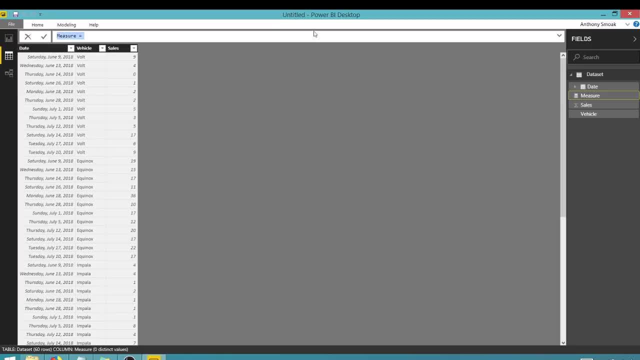 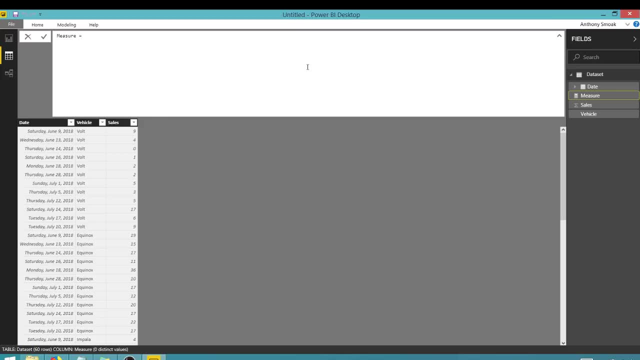 going to go to the data. I want a new measure, and we have to write a calculation in DAX, And so DAX it's a formula language, not a programming language. It stands for data analysis expressions And it's basically a library of functions used to build formulas and expressions. 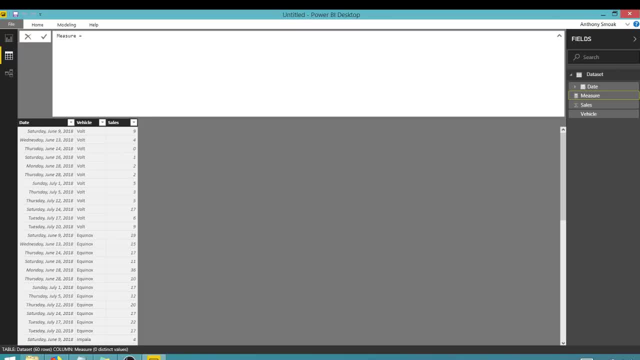 So fortunately, or unfortunately, you have to know some basic DAX to be effective in uh in Power BI. So how do we get that, uh, that percent of total? So I'm going to start out by using this uh divide function. Uh, I'm going to go to the uh, uh, uh, uh, uh. 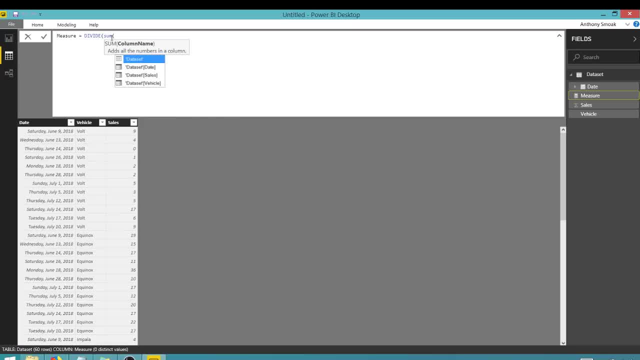 divide function and I want to sum the number of sales right, And I'm going to use this calculate function. So this calculate function is uh, um, it's a pretty useful function in, uh, in DAX here. Um, it's um, you, you enter calculations then then you enter a. 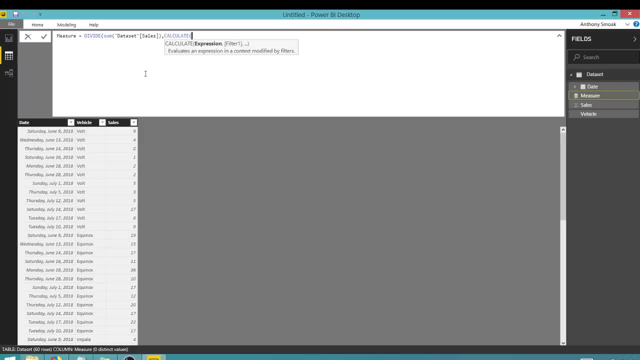 filter expression for that calculation right. So what do we want to calculate? We want to calculate the uh sum of our sales right And then, um, our filter is going to be. I'm going to use this all selected function. 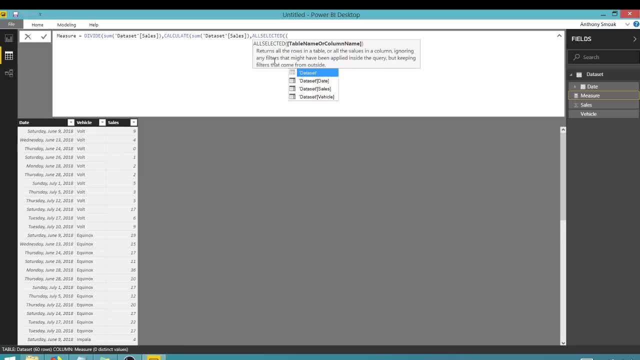 And I'll explain what this is doing. uh, later. and all selected on the dataset, Close the all selected. uh, we're closing, Yeah, we're closing the dataset, closing the all selected, closing our calculate, then closing our divide, right, so hopefully that will take. oh, let's call this the um. 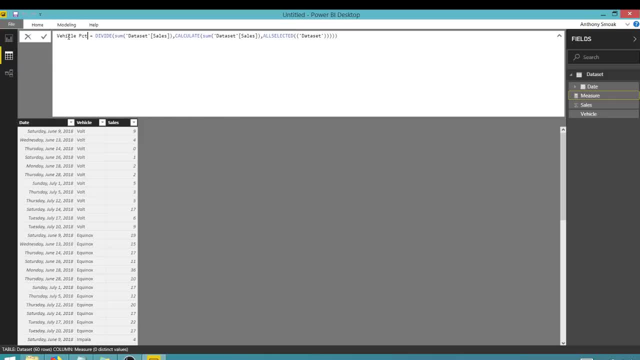 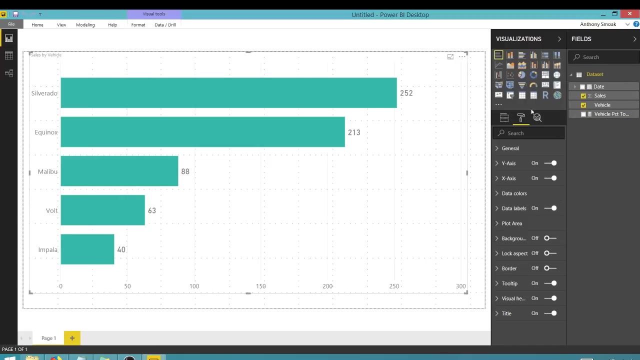 vehicle percent of total sales sales. good enough, get this check. and my syntax is incorrect because i have. let's try that. there we go. i had an extra parentheses apparently, so if i go back here and i look at this vehicle percent total, i'm going to take off sales here and we're going to put on vehicle percent total. 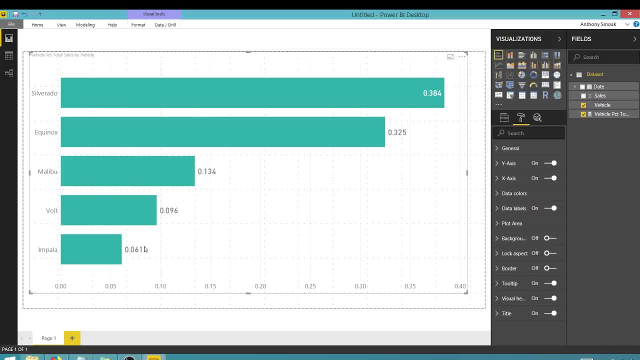 you'll see now i've got a, a percentage. all right, great. and what? what i want to do now is we're going to go here and let's go to modeling and i can hit this percent right and that'll give me a percentage. so so that's how we get a percent of uh total on our bar chart. so let's say i'm going to uh. 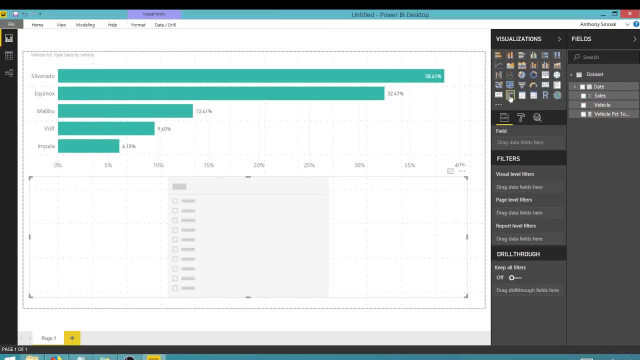 size this up a little bit and i want to put a slicer on here. so you saw that i used that all selected uh function, so let me put the vehicle on here on this slicer and just again, just for visualization's sake, i want to show on the items: let's, uh, let's up the font here, just so you can read this: 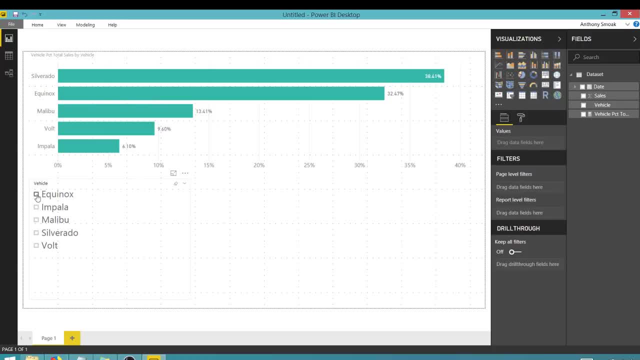 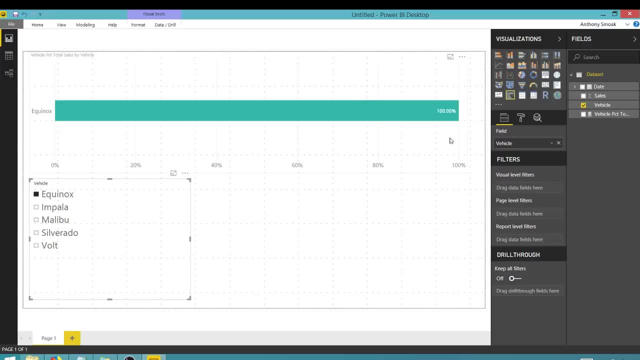 uh, on my different cars. so i'm on, i have all selected. so if i select equinox, you can see that the percentage changed to 100. that's because, uh, i've only selected equinox, there's no other. there's no other selections. uh, the only thing selected is equinox. so if i select impala here, uh, for eze. 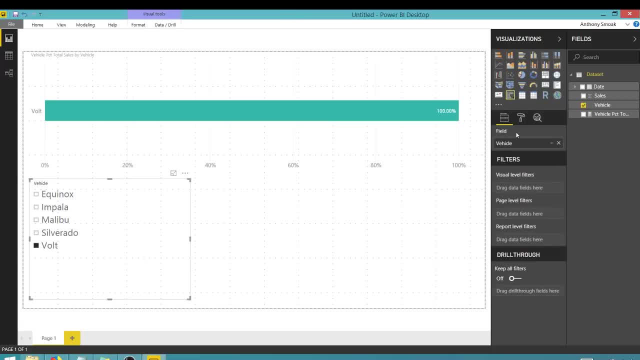 well, let's do this. first let me go in here and for uh, for slicer, there's selection controls. i'm going to turn that on. i'm going to turn on single select. i'm going to turn that off, right. so now i can choose. i can choose equinox, right, i can choose impala, and you'll see that the 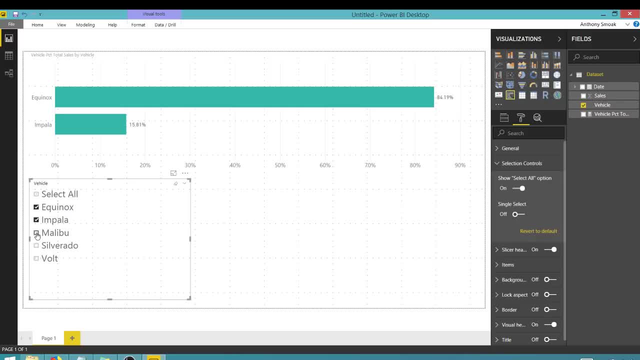 percentages change based upon my selection, so i'm going to turn that on and i'm going to turn that on. selections right: Malibu, Silverado and volt right. so now I'm back to all selected right, what I originally had. if I start taking things away, I'll have a 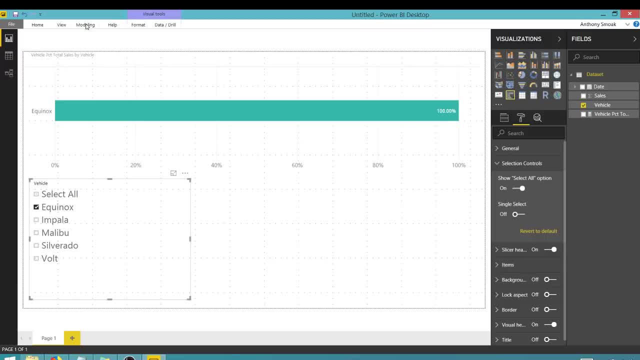 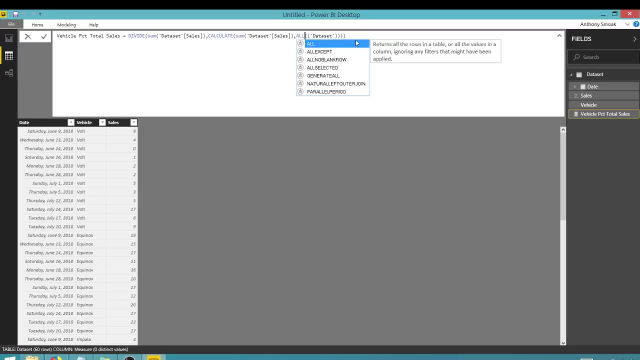 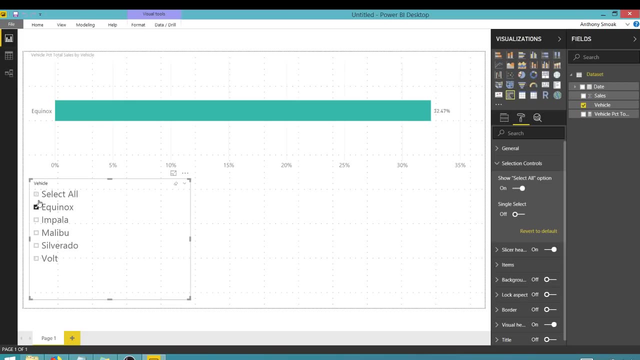 hundred percent. so now if I were to go into- I'm sorry, let's go back here and let's change this to all right and check here all right. now see how my equinox it's no longer 100%, it's 32%. if I bring an impala, 6%. so my total percent. 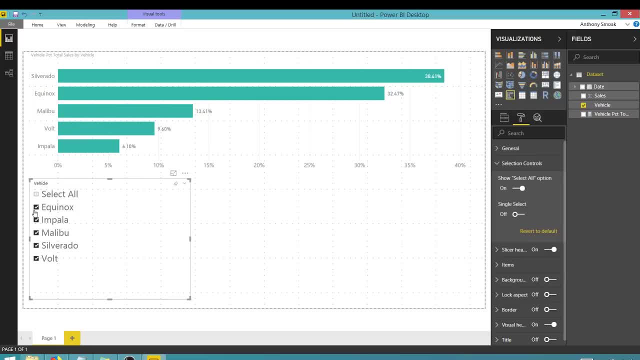 here stays the same, it's, it's static, no matter what selected. when I, when I have all as my filter criteria, use that in the filter criteria right, whereas if I use all selected, that percentage is going to change based upon what is selected. so know that, know that. 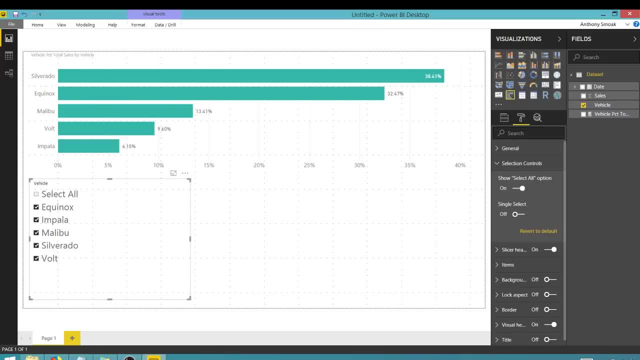 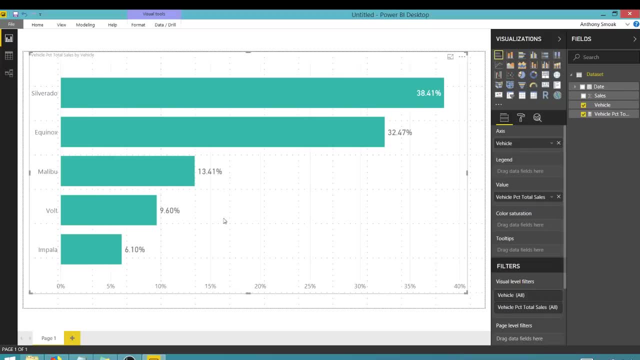 difference when you're using this, this calculation, right? so let's get rid of, let's get rid of our filter. bring this back out. and just another couple things here on on coloring, right, so let me take, let's take sales and and bring that over to color saturation and as you can see, all right, I can get, I can. 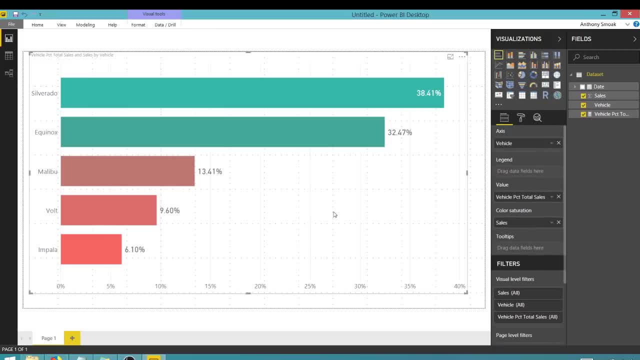 change these, these colors here because I may not like green and red. so if I go into the second tab here for format, I can go to data colors and I can change the colors here. so for minimum, you know, maybe I, maybe I keep it in the the green. 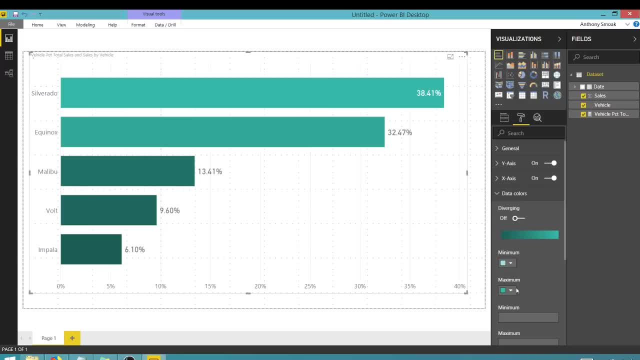 spectrum here. well, let's make it light green, right. and then, for maximum, you know, we'll go ahead and go a dark green there, right. and if I wanted to make it diverging, right? Oh, the center. let's make that center white, right, I can do that. so. 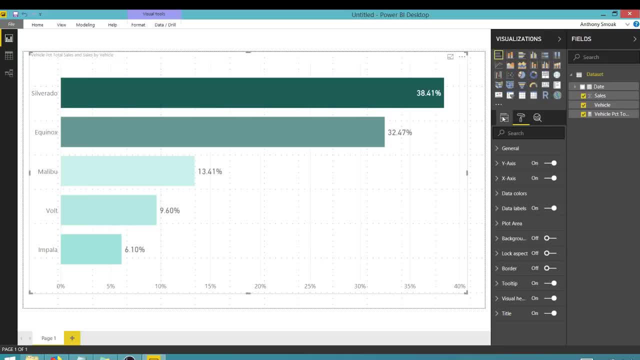 that's how I change the colors here for a diverging. if I go back now, you have to make sure that you have this a value here- sorry, under color saturation- in order to get this option to show up under Diverging Data colors, to get that diverging option to show up. so once you take this away, 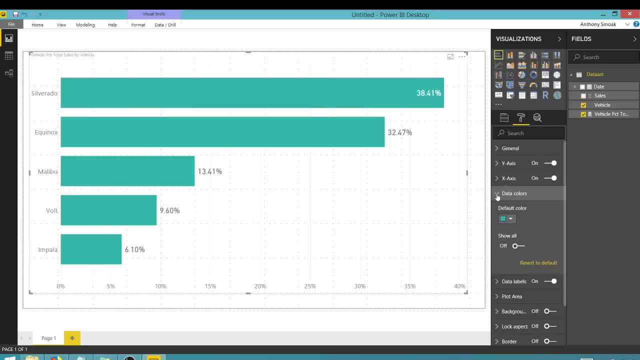 from color saturation and go back to your data colors. you'll see that you don't have that diverging option. but what I can do here, the default option is I can individually change colors here if I wanted to, right. so I can make Silverado red Equinox. you know this is not going to be visually appealing, but 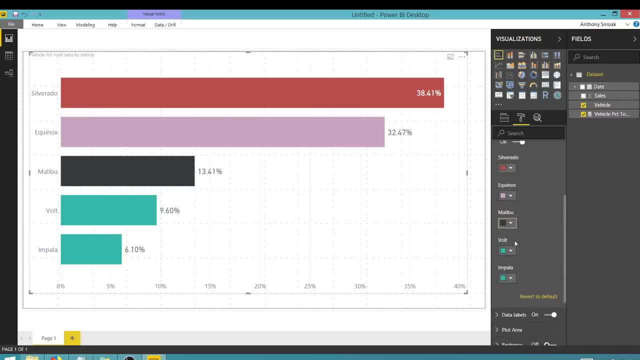 just wanted to show you that it is something that you can do right. so on, so forth. I could change all of these if I wanted to. so again, some bar chart basics here when using power bi. this is the video I wish I had when I started doing some visualization. so hope you. 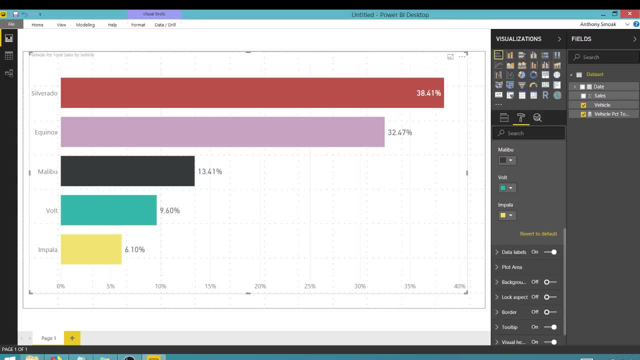 enjoyed this tip. get out there and do some great things with your data. thanks for watching everyone.